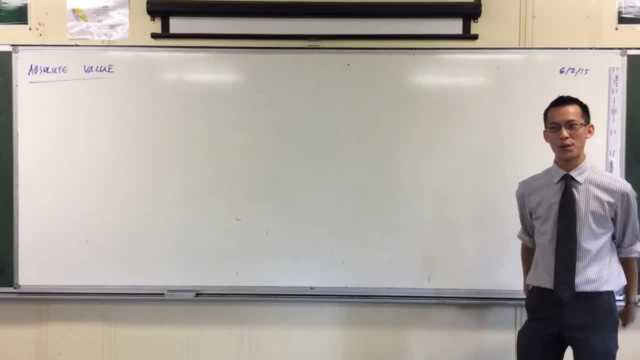 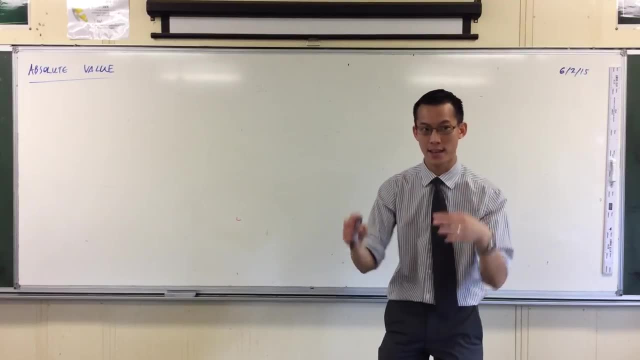 So let me define for you what Absolute Value is. I'm going to give you a variety of definitions that go from sort of simplest, most common sense, and then I'm going to sort of filter down into more complicated abstract definitions. okay, 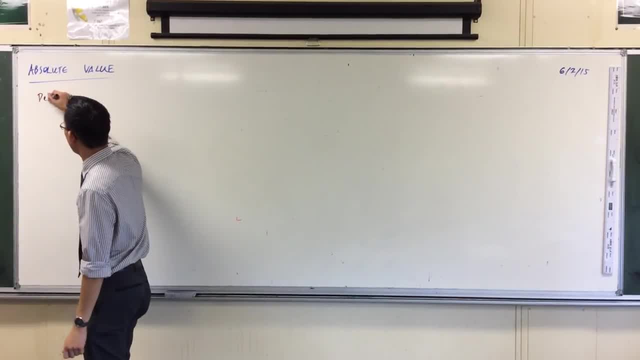 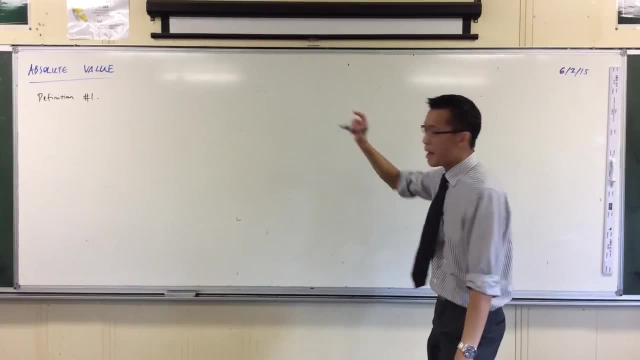 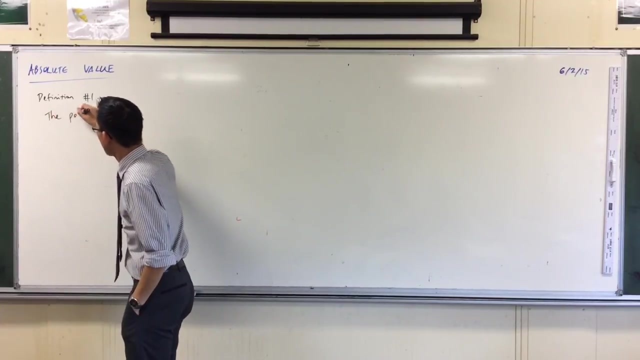 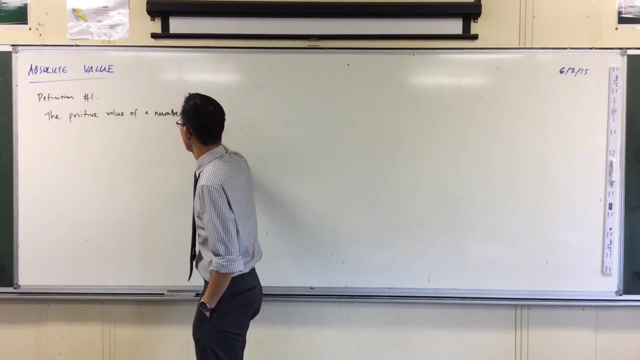 So here's my first definition. Definition number one. Okay, definition number one: Absolute Value- and this is kind of where the name comes from- is The positive value of a number. That's it, The positive value of a number? That is the simplest definition I can give you okay. 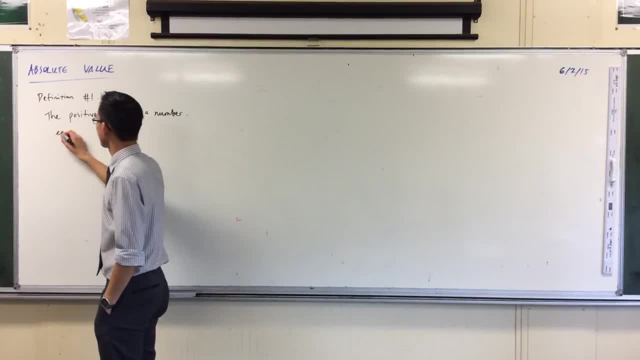 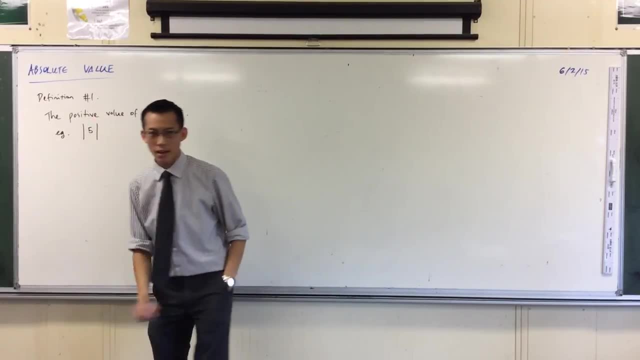 So examples: What does this mean? If I say what's the absolute value, and here's the notation for you, It's two long lines, kind of like parallel lines. you know, it's like those two markers, but separated. 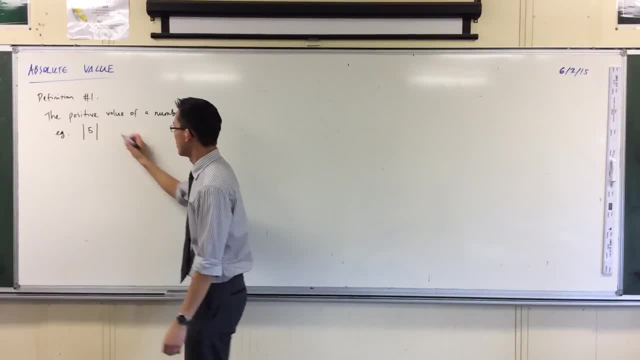 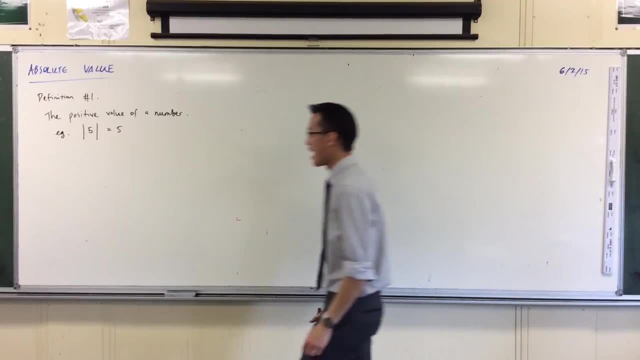 The absolute value of five- that's how I read that out- is equal to five. Whoa mind-blowing. I told you I would start with a simple one. okay, Let's go again. How about the absolute value of negative three? Now, I just want the positive value of that, okay. So therefore it's three. 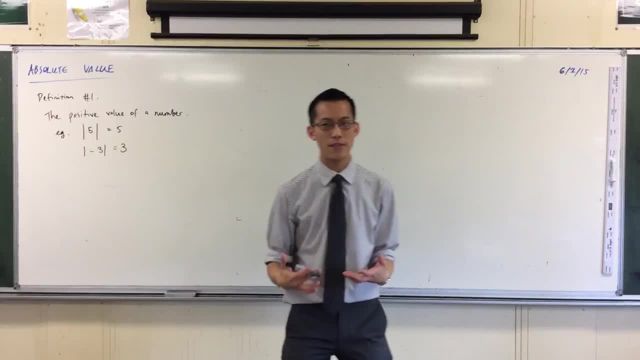 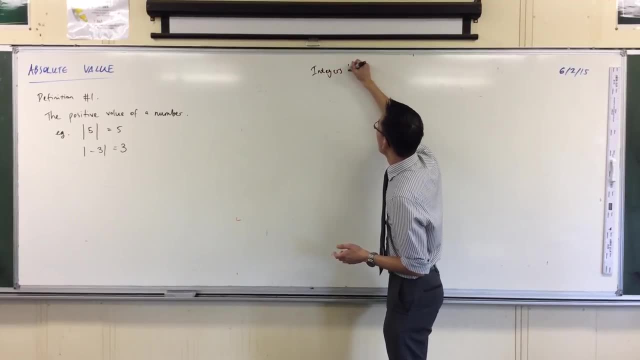 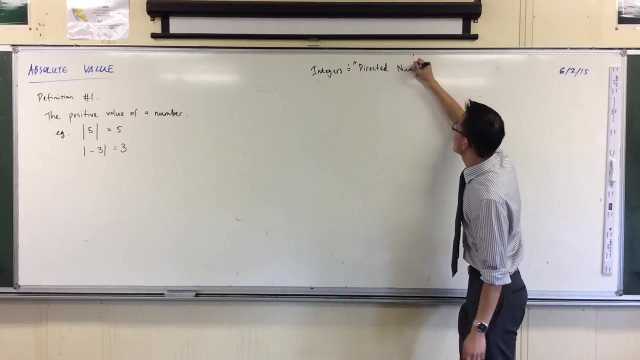 When you are first introduced to negative numbers in the topic of integers in U7, okay, we call integers. Another name for them is directed numbers, Directed numbers, And this idea is important because it explains that numbers they start from just counting right. 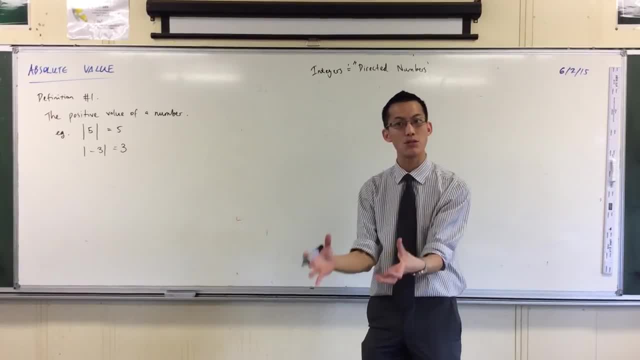 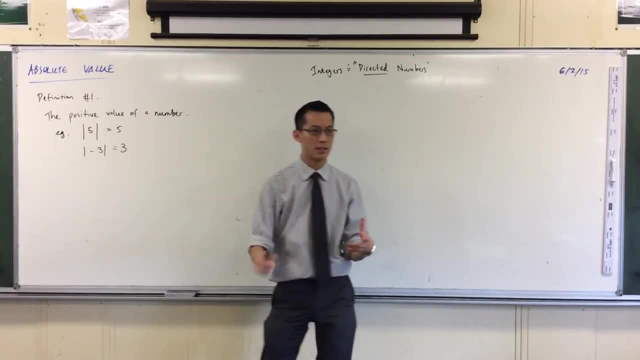 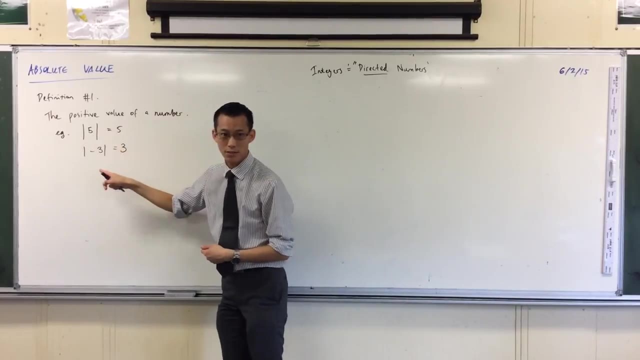 And thinking: how big is something or how much of it do you have? But then it expairs this idea that numbers are not just about quantity or value or size. They can go in certain directions. okay, Integers can go in one of two directions: Positive or negative. okay. 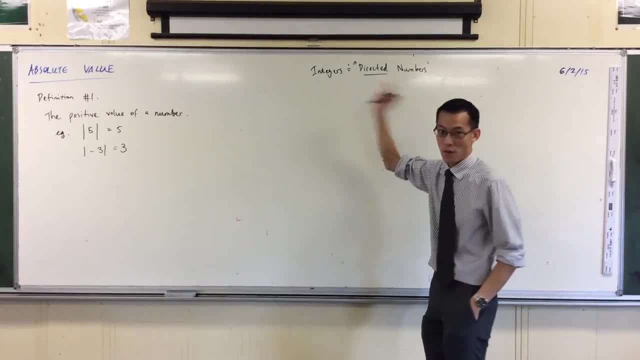 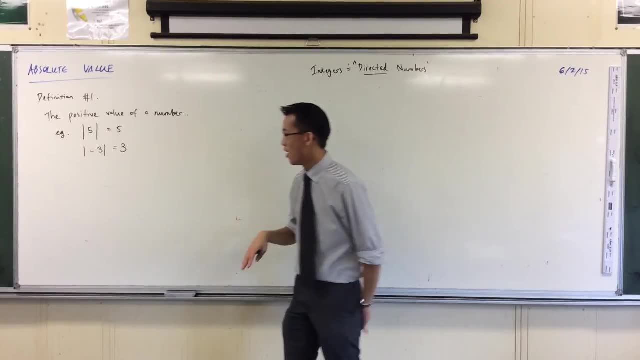 So another way of saying this is: what's the positive direction equivalent of whatever number you're giving? Okay, So positive value of a number. that's pretty simple. You can put these together in operations. It's not that complicated. 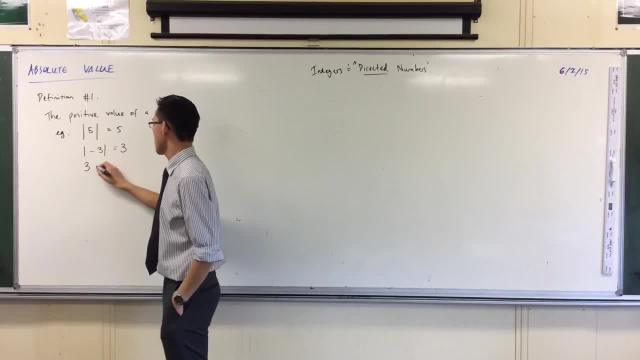 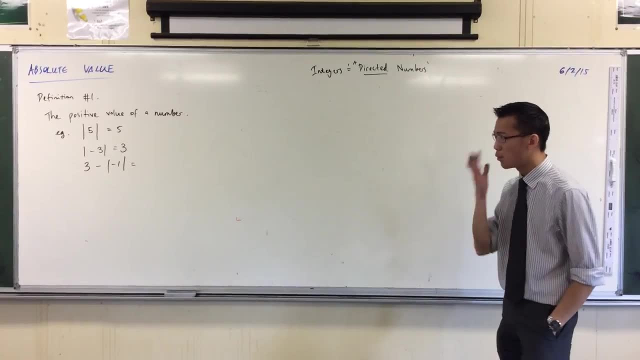 Let's think about this, for example: Let's do three minus, there we go. Three minus the absolute value of negative one, And, by the way, this is something that should have been mentioned to you throughout your years, since you learnt what integers are. 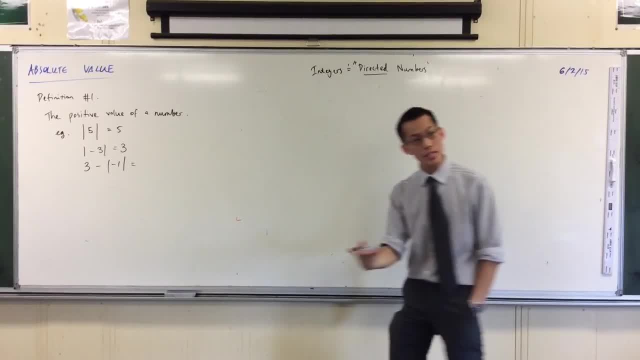 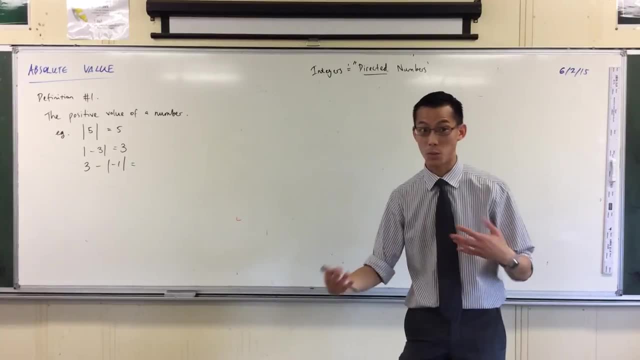 And, by the way, this is something that should have been mentioned to you throughout your years, since you learnt what integers are, are okay, but there is a difference between this minus sign and this minus sign, even though informally, we kind of say three minus minus one, right, and we'll even call that minus one. 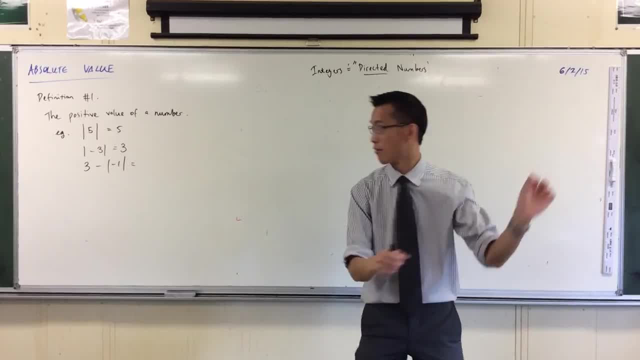 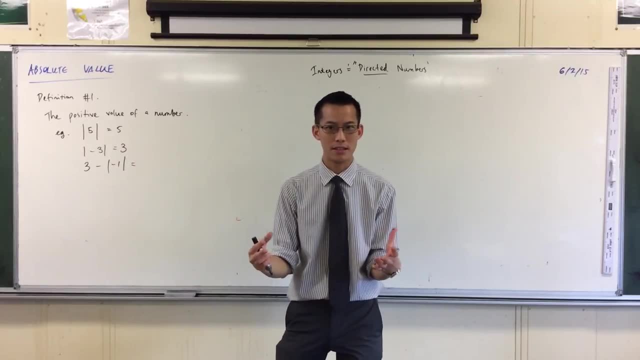 minus is an operation. it says do something right. but here, like this negative number and this negative number, they're actually meant to be adjectives, not verbs. it's it's trying to describe that number and in fact, your calculators even distinguish between these. if you get your. 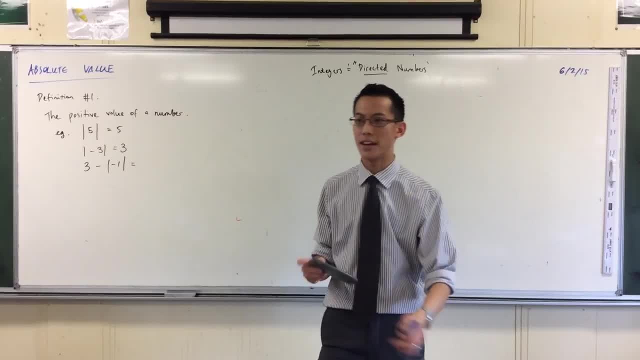 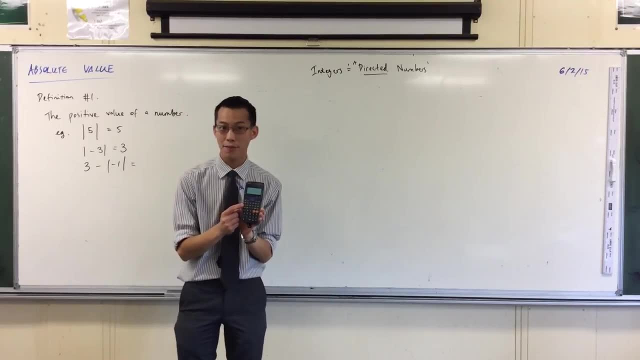 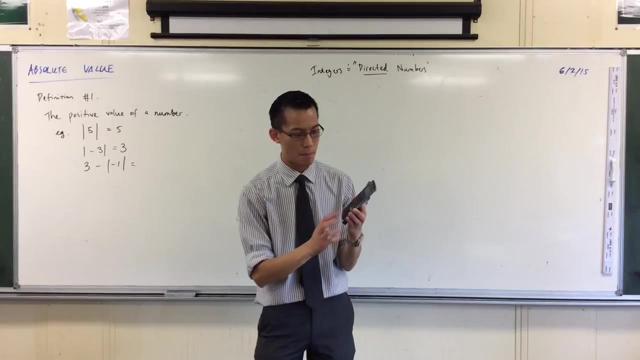 calculators out now. your calculators actually have a negative button on them. you should find it. at least on mine it's on the left hand side. it's a minus sign, a hyphen in a pair of brackets. okay, so when you put that on you might see you get a short hyphen as opposed to the minus, which. 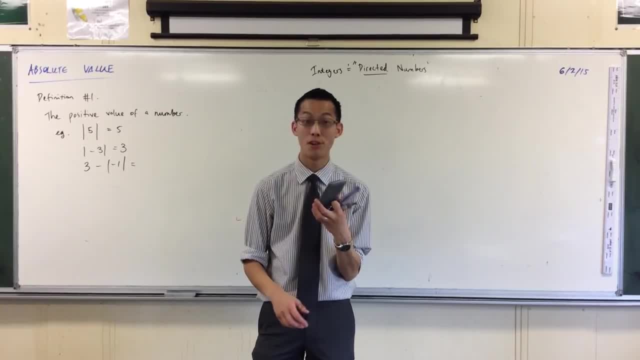 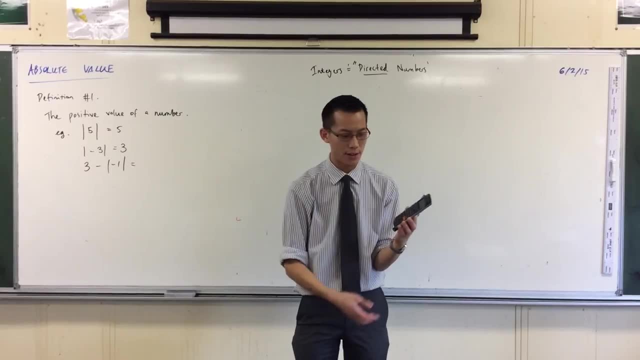 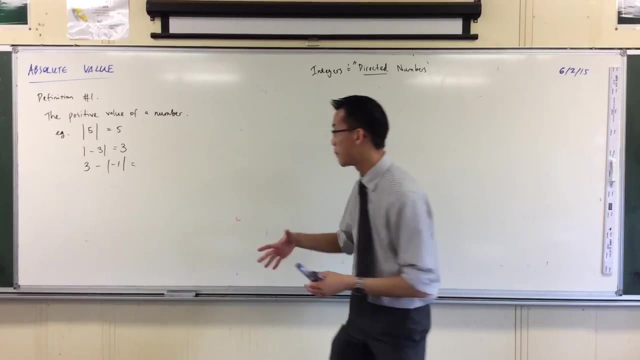 is a slightly longer one. it's like two whole pixels longer on my screen. okay, so there's a minus button and a negative button now, because so many people don't really get that. there's a difference. your calculator, you 'll kind of get what you mean. okay, but let's try now because it's so important to this idea. 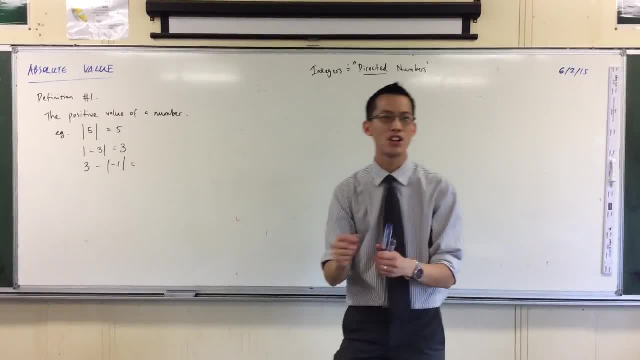 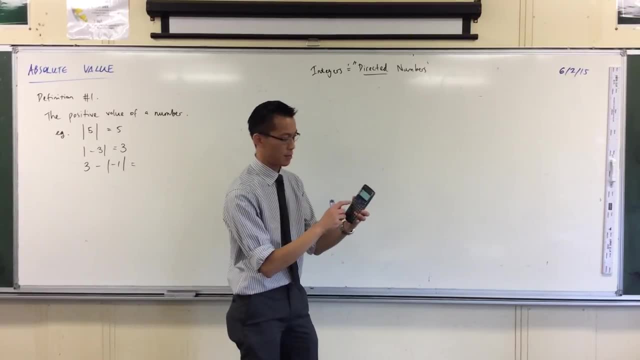 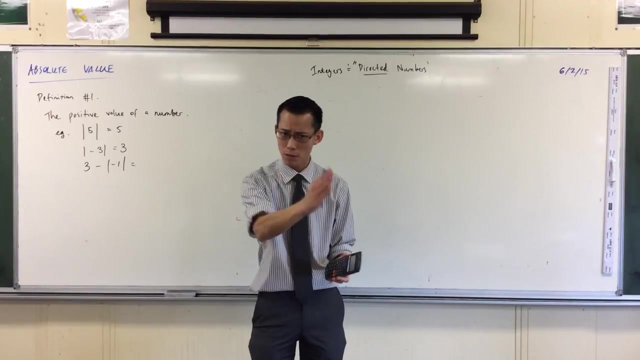 let's try to be a bit more specific and accurate with our language. well, the difference is not all that much, though. if, for example, i just i haven't tested this- but if i go three and then negative one, it'll say syntax error, because negative is not an operation. right, you need an operation. 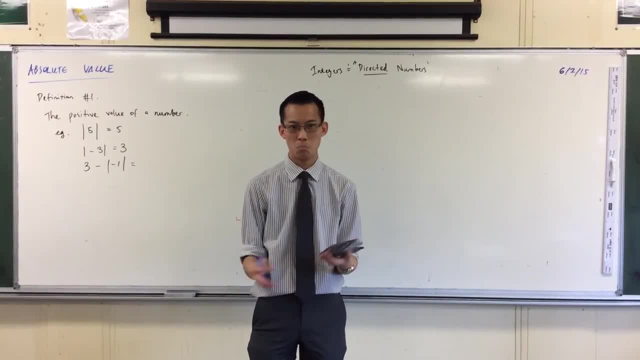 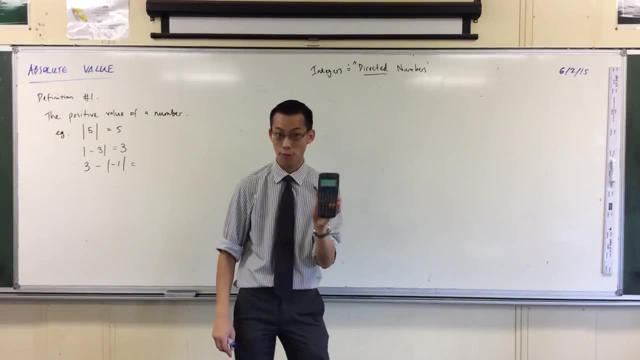 between two numbers and three. negative one has the what's the thing? that's the thing, that's the thing between them, right? does that make sense? so, for example, you could say three minus negative one, and that should give you four, as you expected. positive four. all right, so now coming back to this, 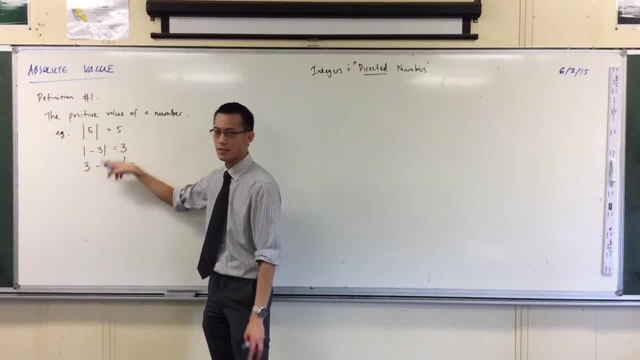 so i'm going to read this out as three minus the absolute value of negative one. okay, it's a simple example, so we'll just like any other kind of brackets, we'll just go from the inside out. three minus what's the absolute value of negative one one. so this is two, no big deal.